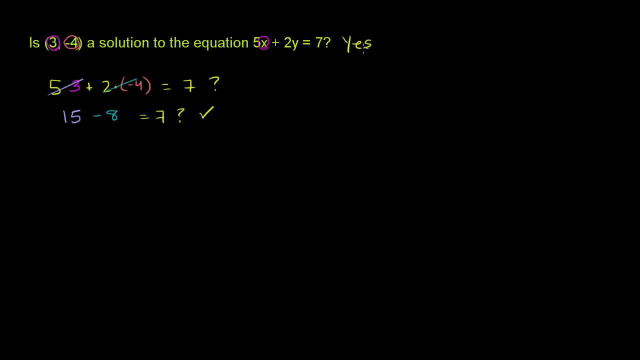 So this all works out. This is a solution. So we've answered the question, but I also want to show you this way. we just did it by substitution. If we had the graph of this equation, we could also do it graphically. 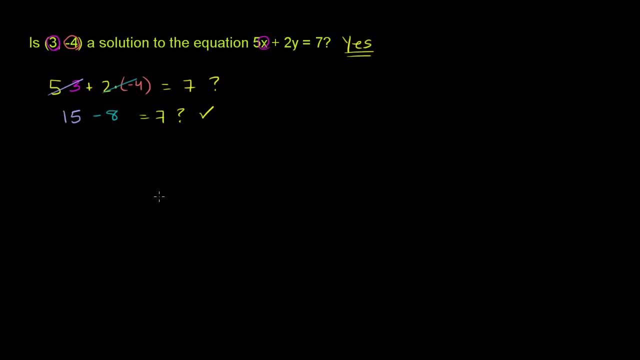 So let's give ourselves the graph. I'll do that by setting up a table. There's multiple ways to graph this. You could put it in a slope-intercept form and all of the rest, But I'll just set up a table of x and y values. 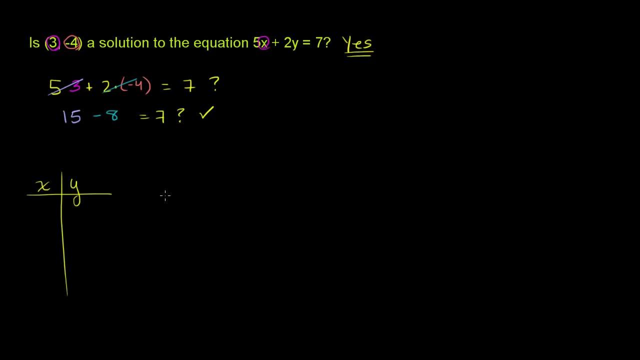 x and y values And I'll graph it. And then, given the graph, I want to see if this actually sits on it, And obviously it will, because we've already shown that this works. In fact, we could try the point 3, negative 4.. 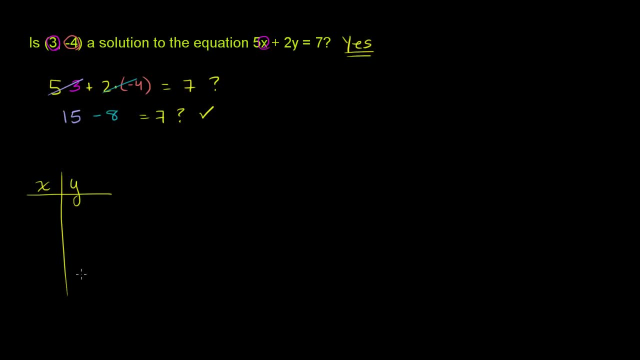 And that actually is on the graph. We could do it on our table, But I won't do that just yet. I'm just going to do this to give ourselves a graph. So let's say, let's try it when x is equal to 0.. 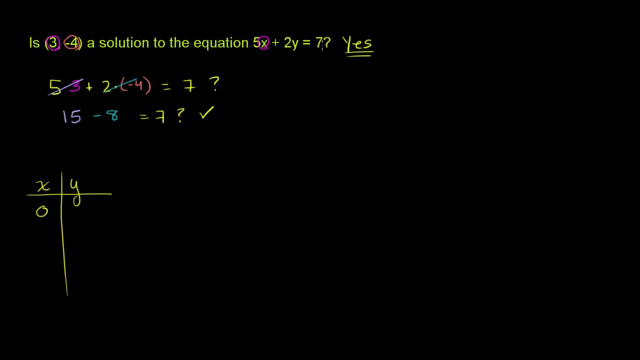 We have: 5 times 0 plus 2 times y is equal to 7.. So when x is equal to 0, y is going to be. so you're going to have: 0 plus 2y is equal to 7.. 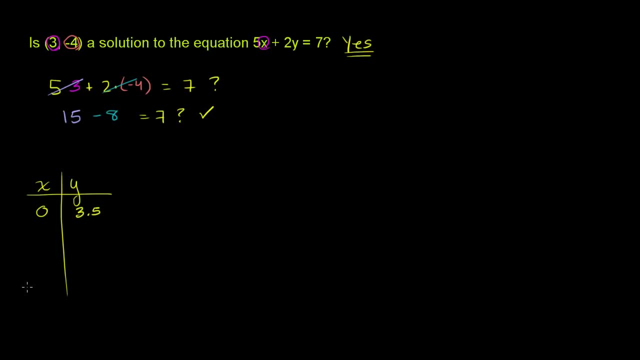 y is going to be equal to 3.5.. When x is equal to 1,, you have 5 plus 2y is equal to 7.. You're going to have 5 plus 2y is equal to 7.. 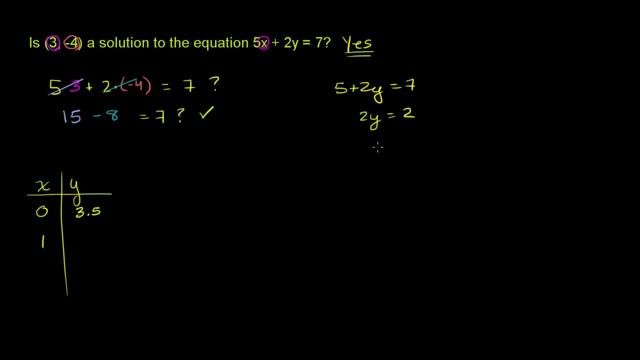 If you subtract 5 from x, from both sides, you get 2y is equal to 2.. You get y is equal to 1.. So when x is 1, y is 1. And when x is well, let's try. well, that's actually enough for us to graph. 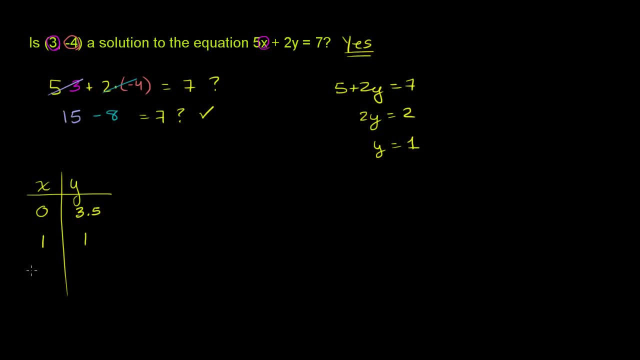 We could keep doing, but we could keep doing more points. We could even put the point 3, negative 4 there, But let's just try to graph it in this very rough sense right here. So let me draw my x-axis. 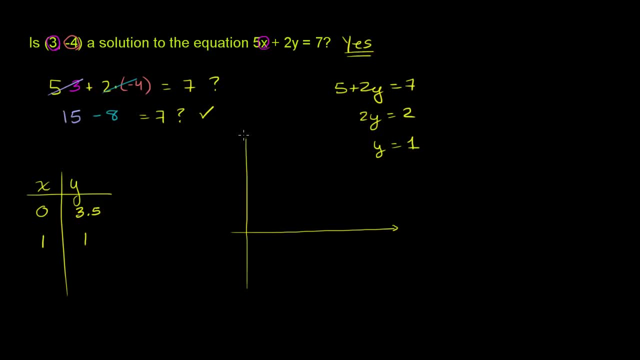 And then this right over here is my y-axis And let me draw some points here. So let's say that this is y is 1, 2,, 3,, 4.. This is negative 1, negative, 2, negative, 3, negative 4.. 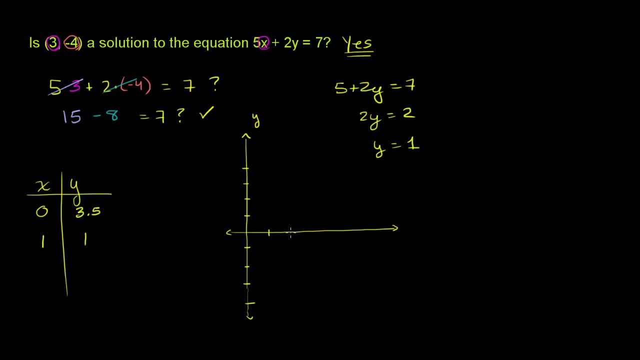 I could keep going down in that direction. This is 1.. Let me do it a little bit: 1, 2,, 3,, 4.. And I could just keep going on and on in the positive x direction. So let's plot these points. 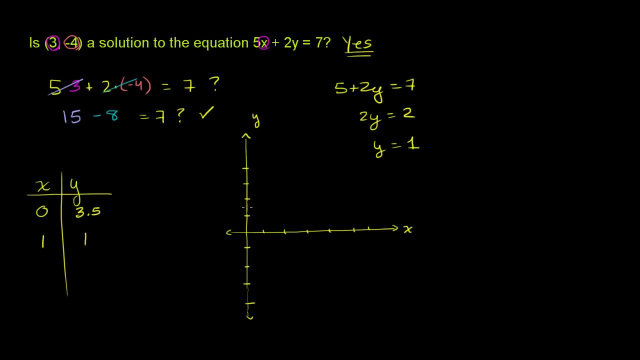 I have 0,, 3,, 4., 3.5.. When x is 0, y is 1,, 2,, 3.5.. When x is 1, y is 1.. When x is 1, y is 1.. 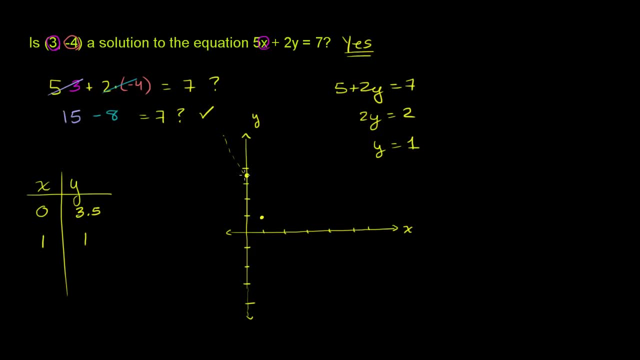 And so if we were to draw this line, I'll do it as a dotted line, just so that I can make sure I connect to the dots. I could do a better job than that, though, So it will look something like that: 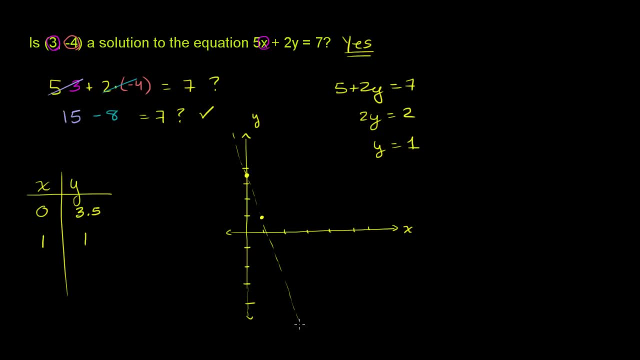 And so if someone gave you this line, you said, oh well, it's 3, negative 4 on this line, And let's assume that we drew it really nicely. And this was all to scale. Let me try one last attempt at it. 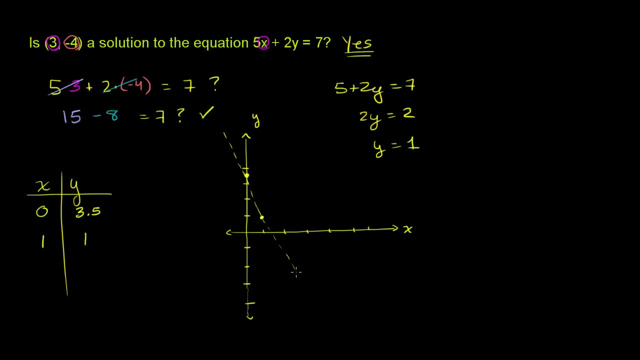 So it's going to look something like that And if someone asks, is 3, negative 4 on it, You could visually do it, But it's always hard when you actually don't substitute it Because you don't know, Maybe you're a little bit off. 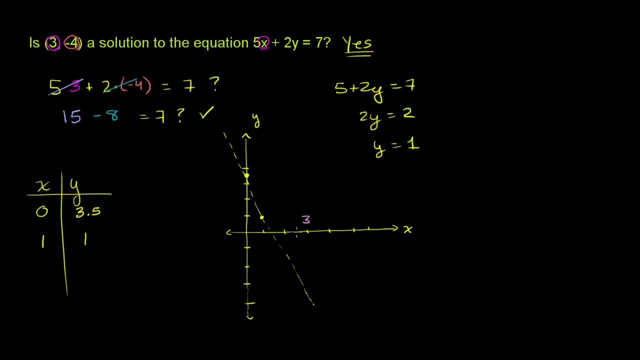 But if you look at over here, you say: when x is equal to 3,, what is y? Well, you go down here and it looks like y is equal to negative 4.. So this is a 0.3 comma, 3 comma, negative 4..